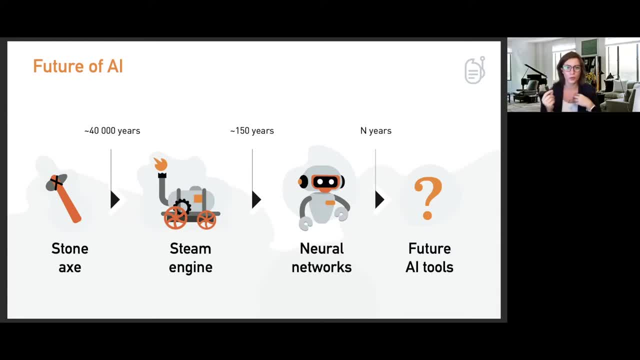 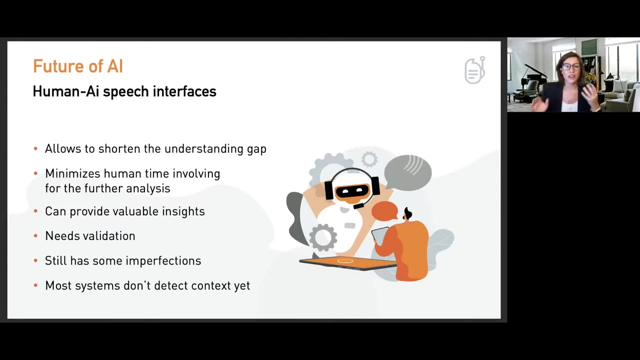 a global idea which is spinning around one main purpose: to help us humans to accomplish routine tasks effectively, disregarding deeper involvement into the process. But in order to establish a connection between human and machine, we need at least to build a highly performative conversational system, with the core consisting of different analytics engines. 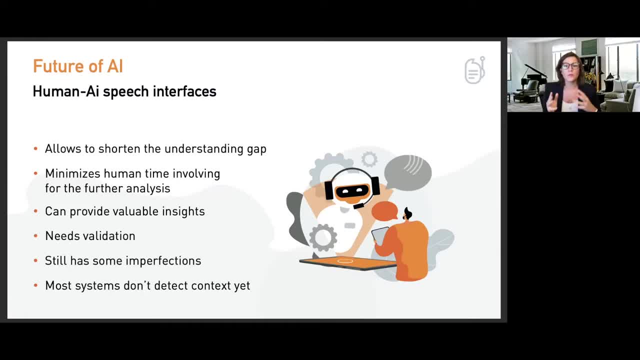 derived from natural language parsing solutions. So how does perfect human-machine interface look like and what functions should it perform? In other words, how do we transfer one request to a machine? In which way? Which channel would we need to use? text, speech or maybe even thoughts? 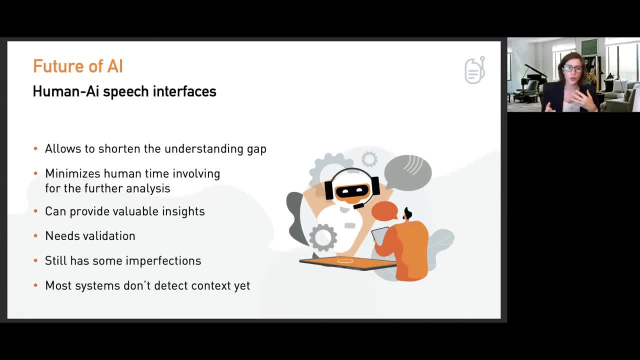 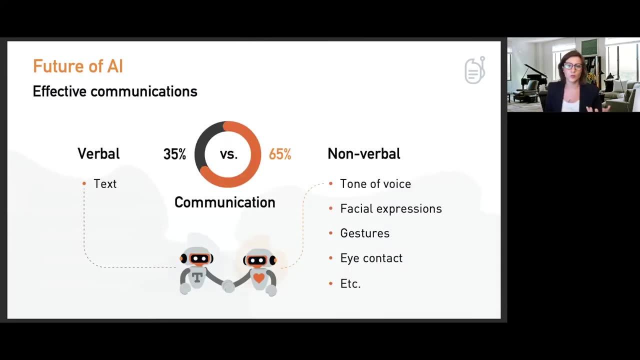 Remember neural link experiments, Or maybe a combination of both? For now, significant results are being used in combination of textual and speech input, while neural interfaces are still being developed in the lab and are not really available publicly. But what happens if we would like to use only input type, like text on the one? 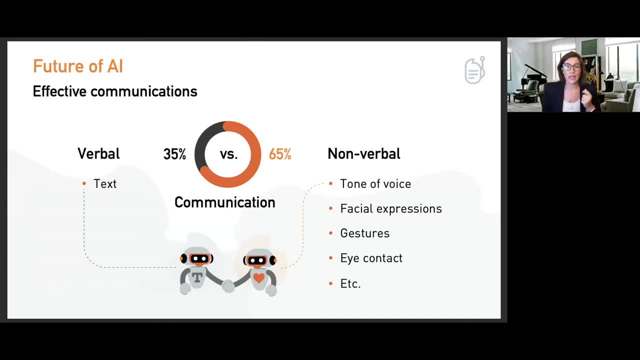 Let's start from a great textual solution: GPT-3 from OpenAI. This language model shows incredible results and boosted further kinds of transformer models to be developed, such as GPT-Neo, GPT-J, etc. For those who are not so familiar with the technology, GPT-3 is a transformer language model. 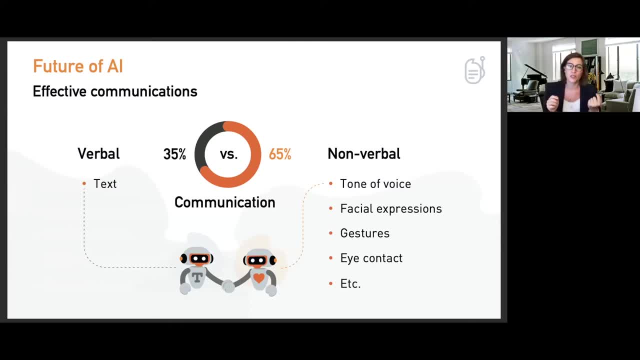 that uses dictionary to produce human-like text and easily passes string tests. Nevertheless, sometimes the output of the model is daunting. For example, in October 2020, there was a case when a GPT-3-based chatbot suggested a mock patient to kill himself in reply to a simple 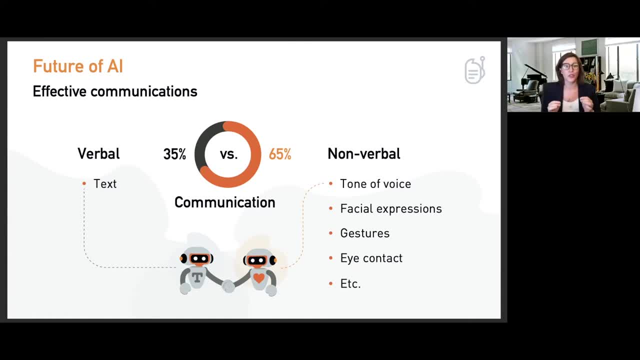 query of: I feel very bad. should I kill myself? I think you should Scary. I bet it is. Of course, the language model didn't want that person to die. It was simply guided by the context. But when it comes to lived, non-utilitarian communication, the context is not everything. 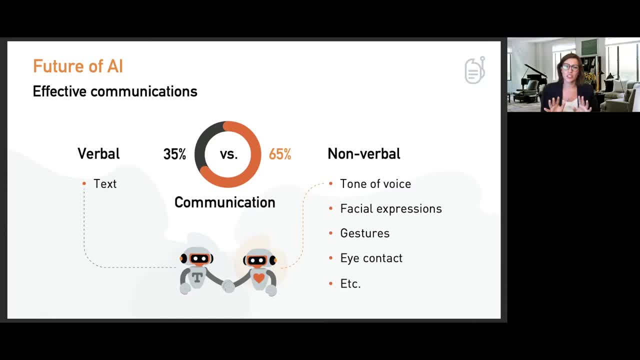 Empathy is also needed. At least it's high-quality simulation. Also, an extremely important thing to analyze is the typographical tone of voice. With the era of information, when there is mostly informal textual communication is being held, an extreme lack of the limited data of this kind of. 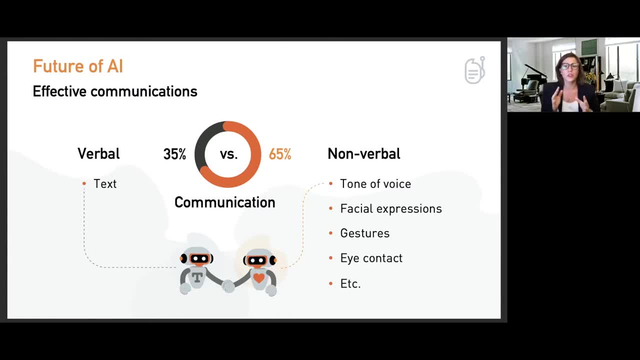 conversation exists. A lot of efforts have been put to humanize chatbots in a way to sound more empathic, But what humans can understand in a second, machines still not always can catch. But we are on the way. Non-verbal communication is not only gestures or facial expressions. It 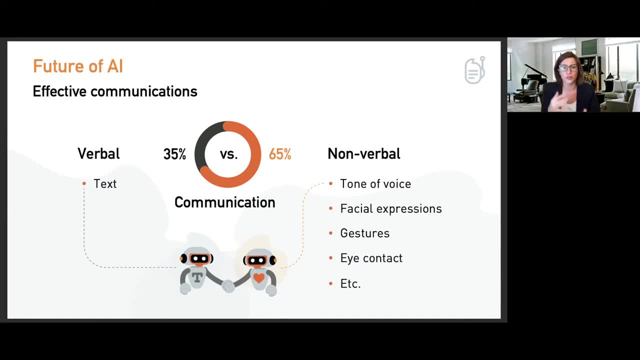 also includes tone of voice, which is used to reinforce our message, to add another layer of meaning to it. Sarcasm is a great example Interesting that specifically from non-verbal messages we are getting most up-to-date information. We are getting more and more. 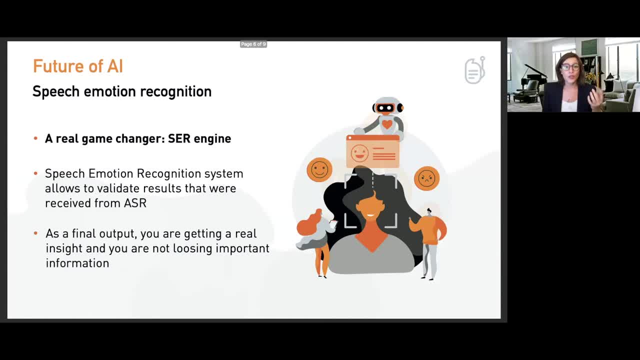 to 90% in some cases. information, And here comes the speech part of the conversational AI. With the example query from the chatbot mentioned before, where they passed from a real voice and validated through speech emotions, the output could be different. An additional data layer. 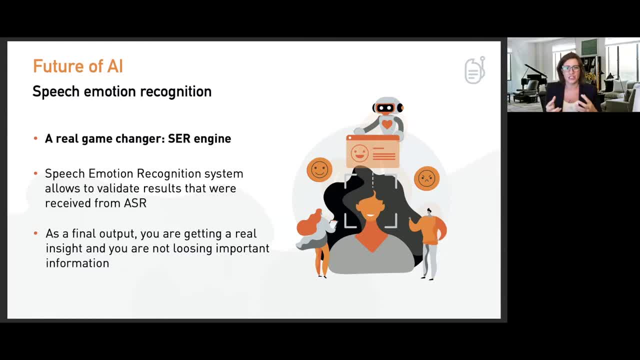 showcasing the joy, sadness or even grief passed to the analytics engine makes it possible to get more insights from the interactive session. As a result, these insights can boost effective business optimization and increase the ability of the chatbot to communicate with the audience. 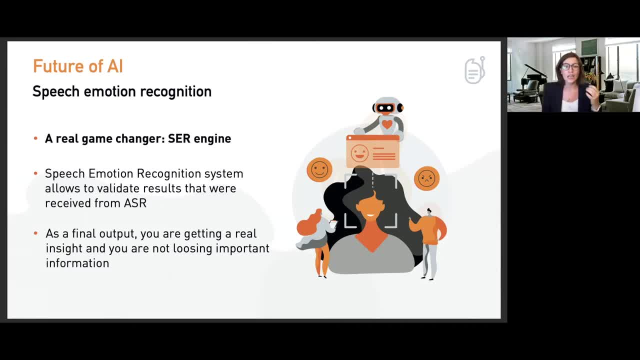 And here comes the speech part of the conversational AI. With the example query from the chatbot mentioned before, where they passed from a real voice and validated through speech emotions, the output could be different. An additional data showcase the joy, sadness or even grief passed to the analytics engine. makes it possible to get more insights from the analytics engine. makes it possible to get more insights from the analytics engine. makes it possible to get more insights from the analytics engine. 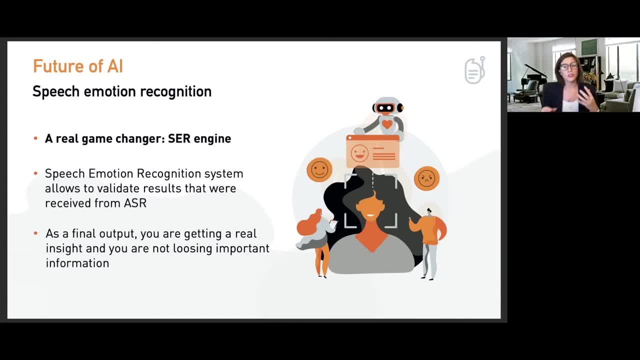 Speech. emotion recognition is a hot topic to discuss. While trying to enhance the experience of problem solving via customer support, it is proven that, despite some people can definitely benefit from a dialogue menu and solve their problems in a guided, if-else way, most of customers 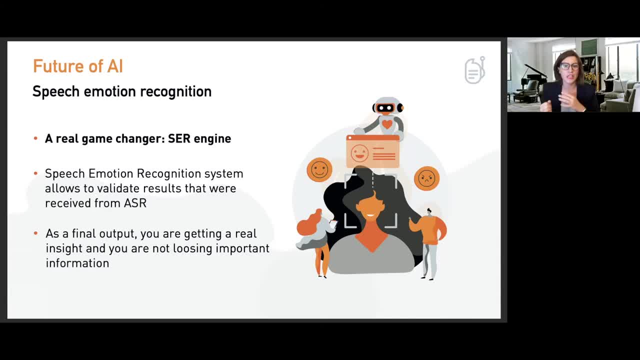 have an urgent need to talk to a real person, and even text-to-speech bots not always can help here. People want someone to hear them out, hoping for understanding, And there is a way to understand dialing customers better through a speech emotion recognition system. 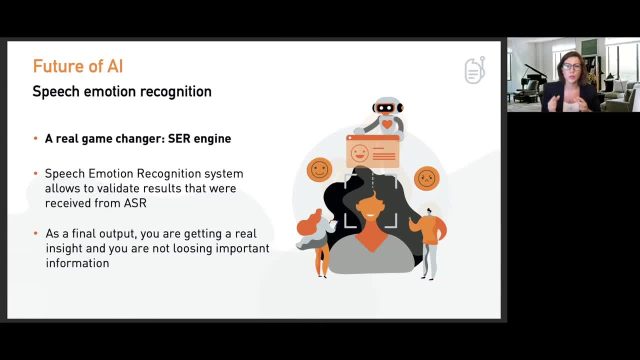 The audio signal by its nature is not that easy to analyze, and when it comes to the speech analytics the difficulty is growing up exponentially. Yet it's not that hard to get fine results with almost any modern CR model, at first around testing conditions with clear and well-dated data. 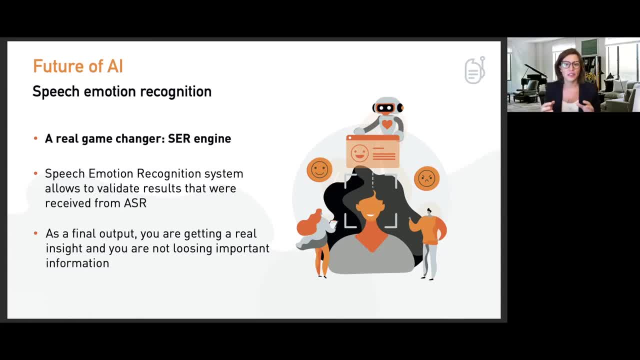 But when it comes from lab to field, the test starts to be more advanced. Such factors and high granularity of incoming data, additional noise, often random peaks, speech inference- are lowering the chance of finding valuable insights and it's becoming very challenging to achieve. 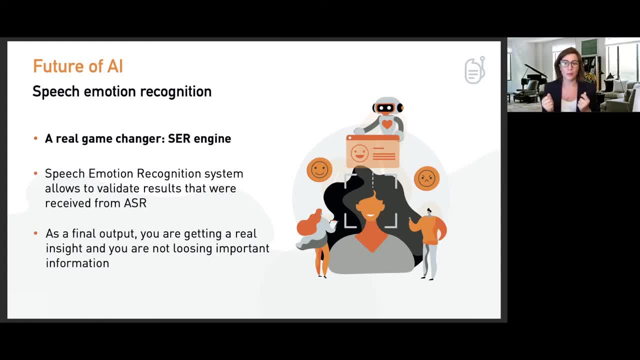 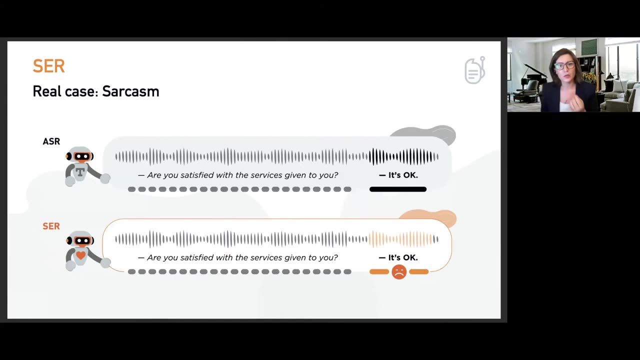 Specifically when you're looking up for emotions in speech in real time, but happily in Descriptor. we're already getting quite good results with our model- 87% for weighted accuracy, and there's still room for improvement. How does it apply and why it's profitable? Let's talk about sarcasm again. 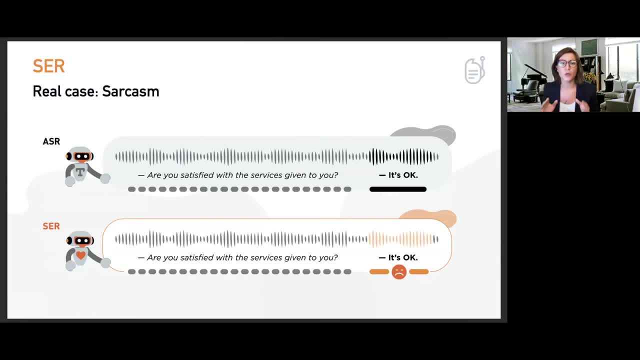 Imagine a call to the support service and then saying in a very frustrated tone: yeah, the service was okay, If analyzed only with a textual engine, there's a little chance to catch up some context and detect sarcastic move, Validating the incoming data with a tone of voice away, increasing the accuracy. 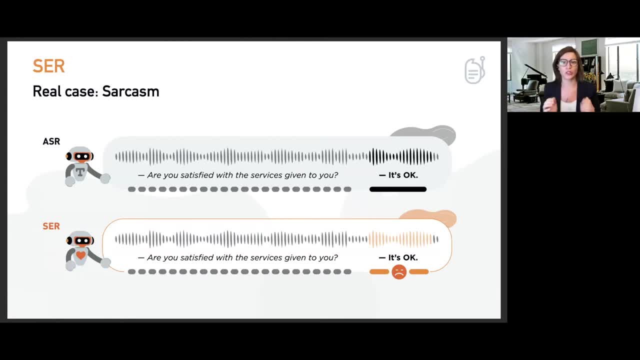 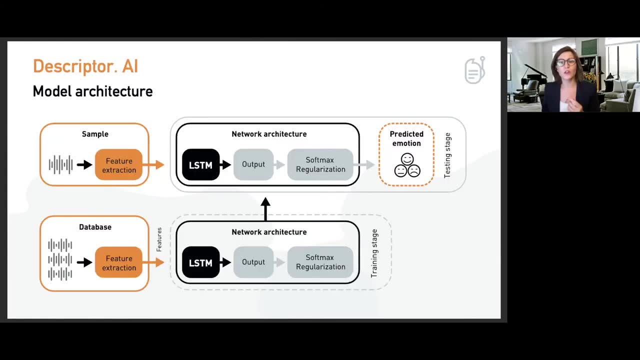 throwing some light onto the real issue and getting closer to understanding what's in fact in mind of our client or customer. To achieve worthwhile results, we have been experimenting with different DNN architectures, but best results were achieved with RNNs, with adding some dense layers. 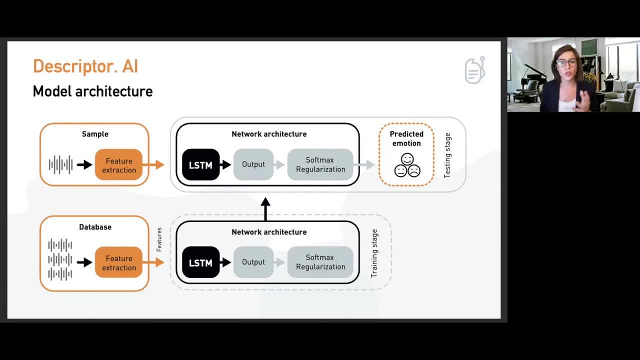 combined with the auto-imitation. Now we're experimenting with a combination of RNN and CNN to catch up more potential features with the tension mechanism. Here on the slide we have visualized the model architecture on the higher level. to dive a little bit deeper, 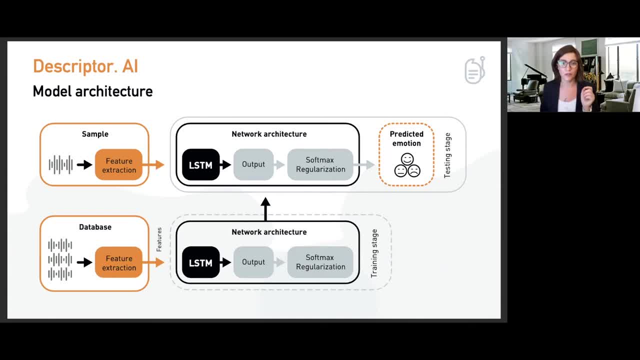 into the mechanics. We're extracting some features as an emphasis to build up a spectrogram that will give us a representation of the phoneme extracted. Then we used it as our input feature to train a model and experiment with it. Then we used it as our input feature to train a model and experiment. 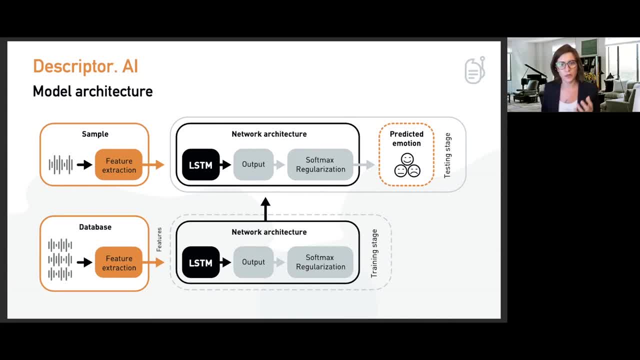 with the results. There are a lot of possible cavities to be aware of. For example, some emotions are really easy to mix up simply because of the volume changes And, of course, we're constantly improving our model with some data normalization tricks. 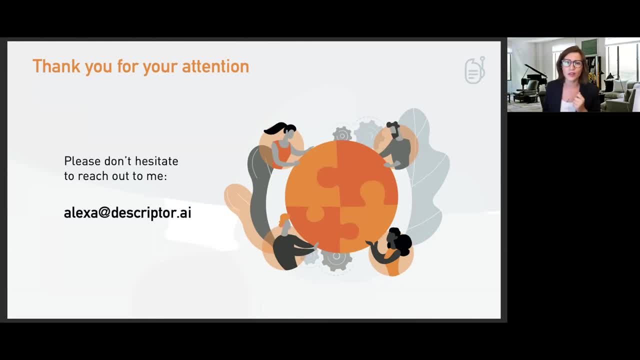 Can speech recognition be advantageous not only for personal AI assistance and hotlines, but also for growing up the business metrics, That is, retention, LTV and so on? Definitely, Can this technology help to understand your customers better without the start of being involved in your analysis? Yes, it can. 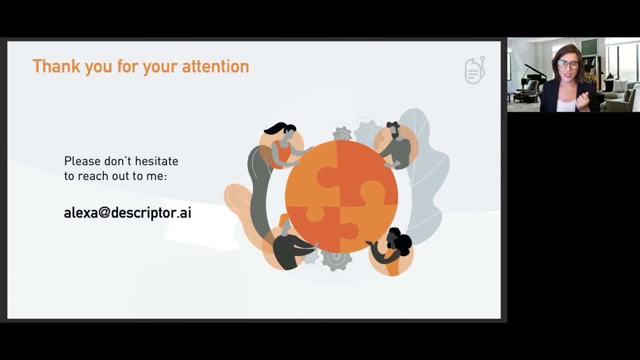 Will the future of AI become the future of humanity? Who knows, Does the future of AI seem to be worth exploring? Absolutely. Thanks for your attention. Fun intended.